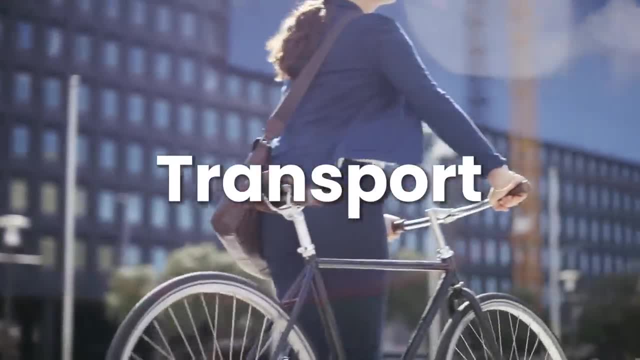 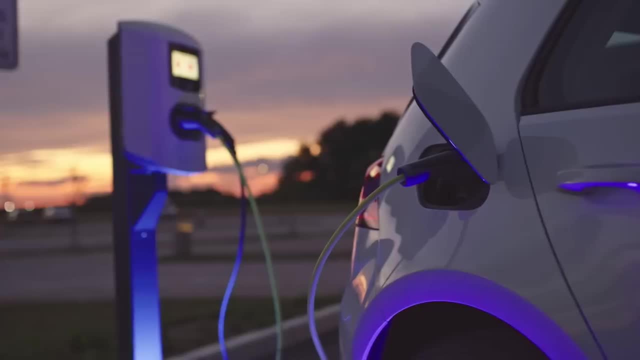 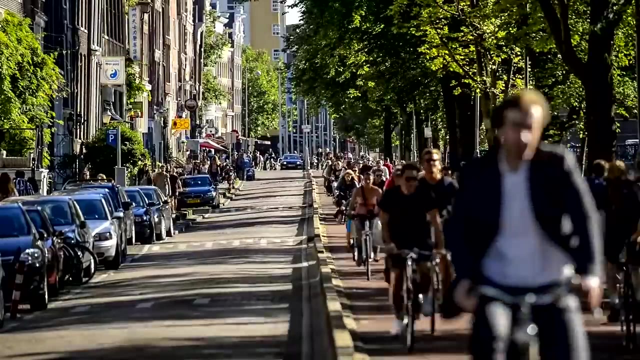 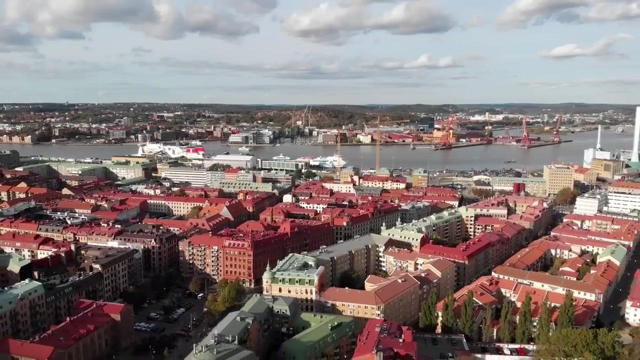 largest changes. As populations continue to grow, cities must also continue to adapt and transform their transport systems, creating access to affordable and sustainable public transport options and creating safer spaces for cyclists. Gothenburg in Sweden is a great example of a city that is dedicated to improving its public transport and creating a wave of green options. 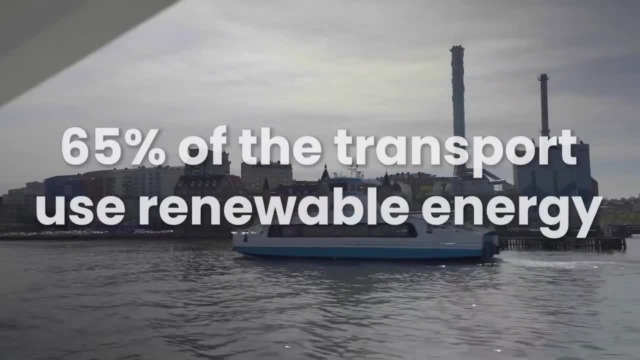 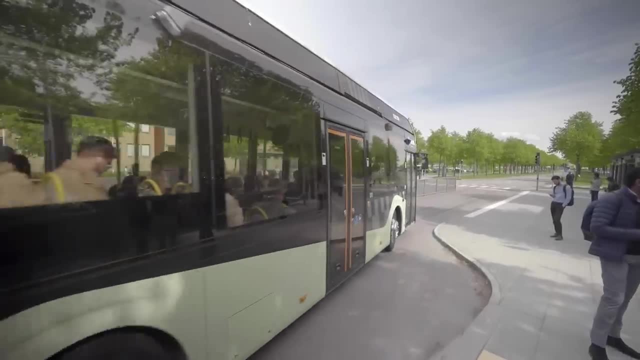 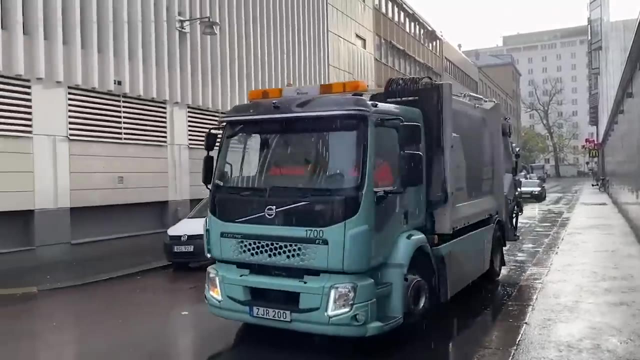 Boasting travel by buses, trains, trams and boats. 65% of the city's transport options use energy from renewable sources, with 200 electric buses serving 34 different routes across the city, as well as electric ferries. Gothenburg has also introduced electric refuse trucks, helping to not only cut down on emissions, 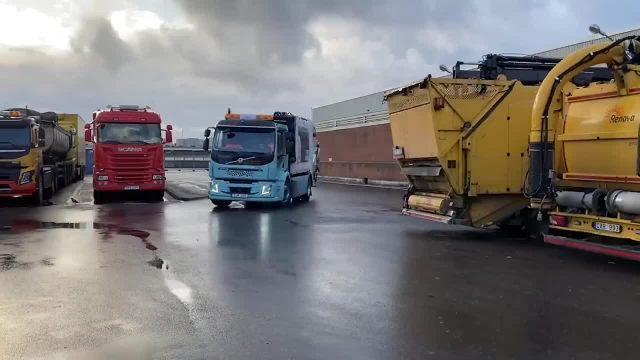 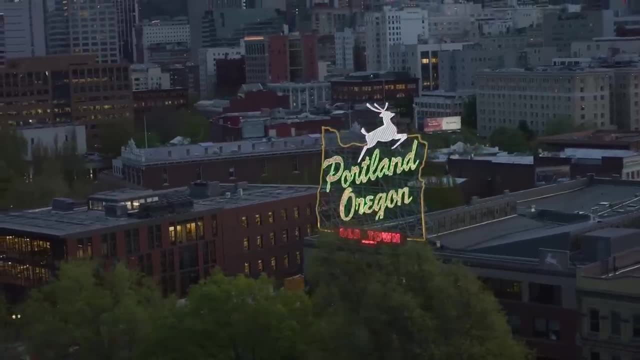 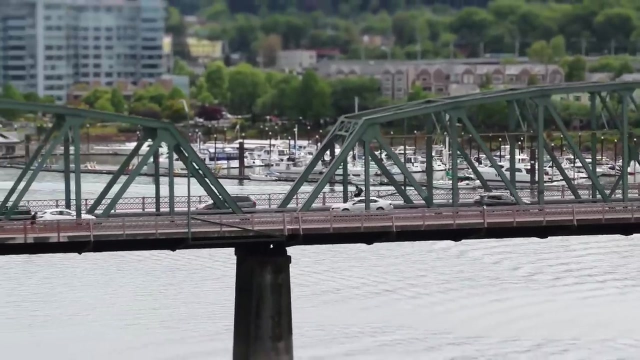 but also lower noise pollution, allowing for less restrictive collection times and, hopefully, creating a cleaner city for all. Another great example of a city promoting green transport is Portland, Oregon in the United States, With over 250 miles of bike paths. 25% of city workers commute by bike, carpool or 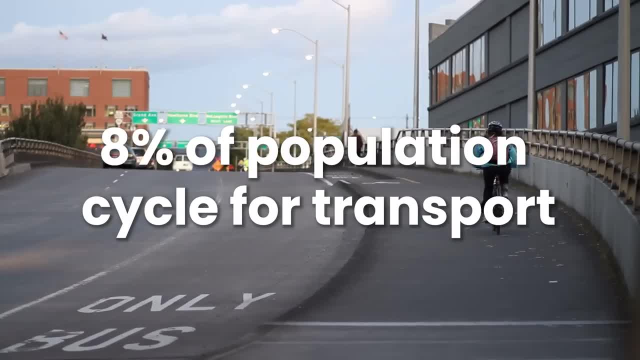 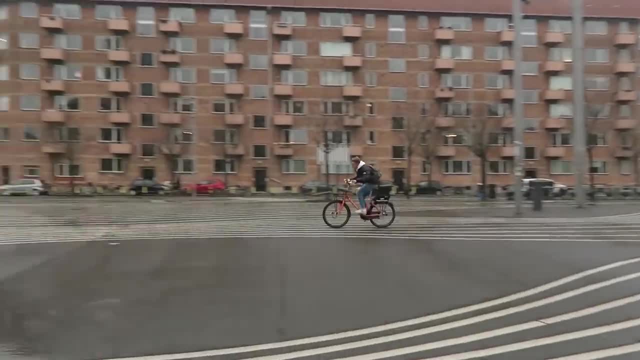 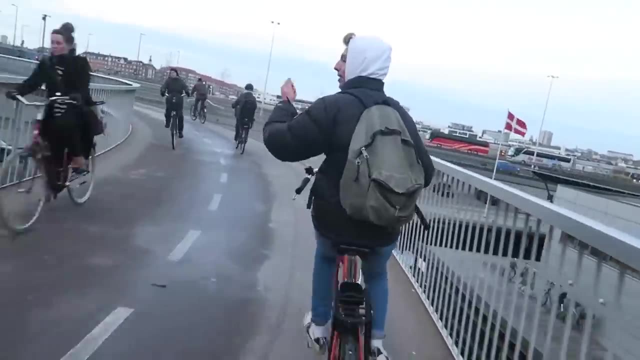 public transport, with 8% of the population using cycling as their main transport method, the highest level of bicycle commuters in any American city. Amsterdam and Copenhagen are also notoriously known for their sustainable transport options, but you can learn more about these two cities in our previous Sustainable Cities video. 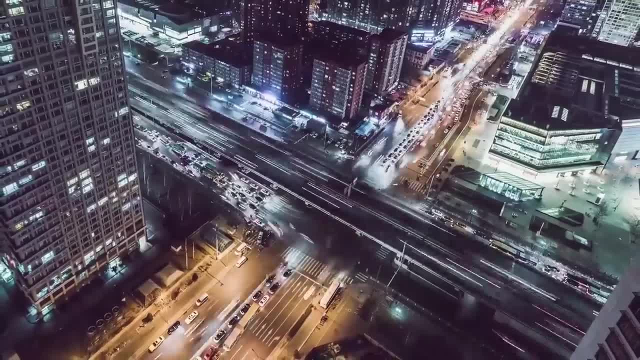 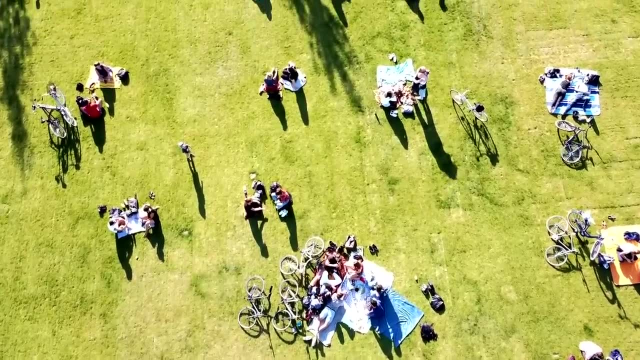 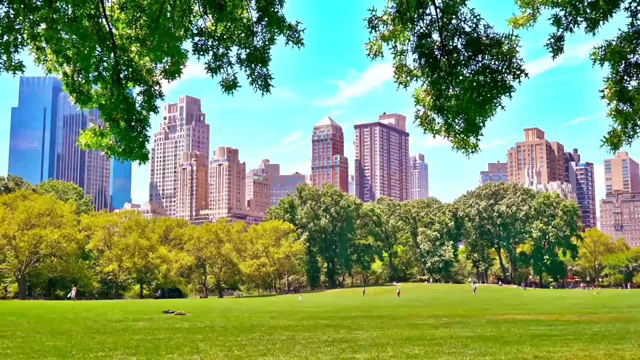 With high amounts of pollutants being generated daily in city centres, it is vital that we find a way to improve our air quality By providing green spaces such as parks, ponds and woodlands. the plant life introduced can absorb carbon from the air, turning it back into oxygen and refreshing our air quality. 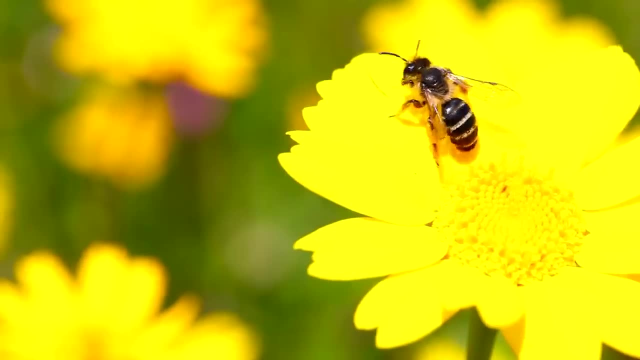 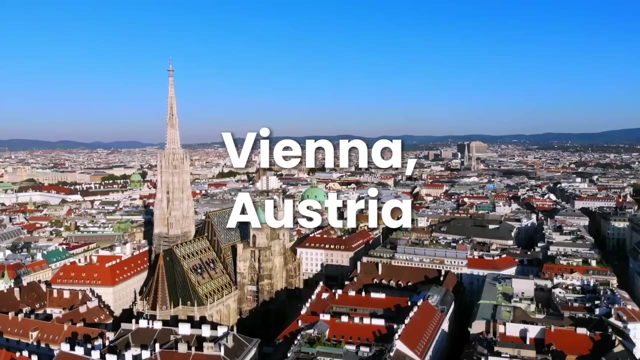 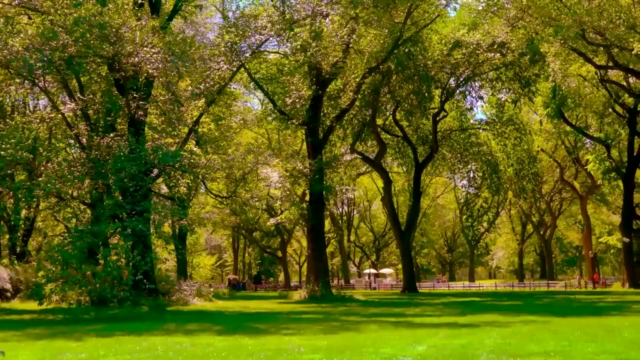 Green spaces also provide a habitat for wildlife, leading to more biodiversity within the city, as well as creating therapeutic spaces for the community and improving mental health. Vienna, Austria, is leading the way for green spaces in cities, ensuring its residents the right to high-quality green and open space that will be maintained in the future. 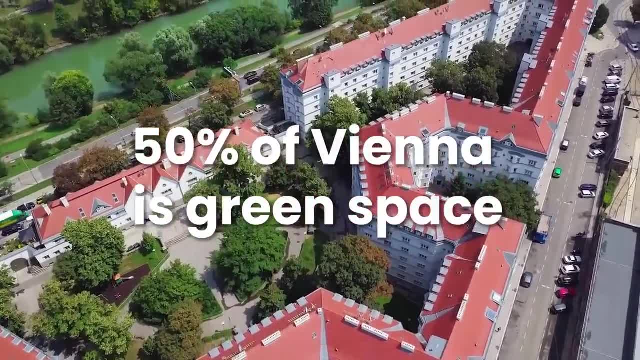 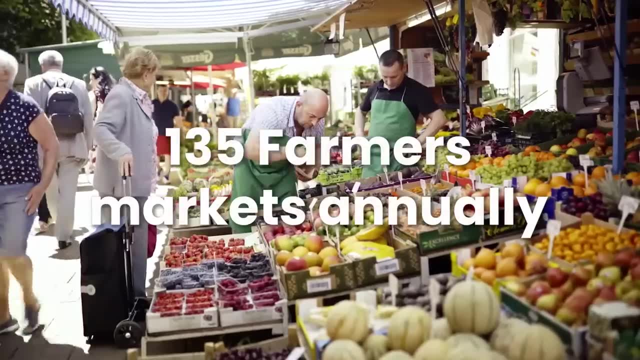 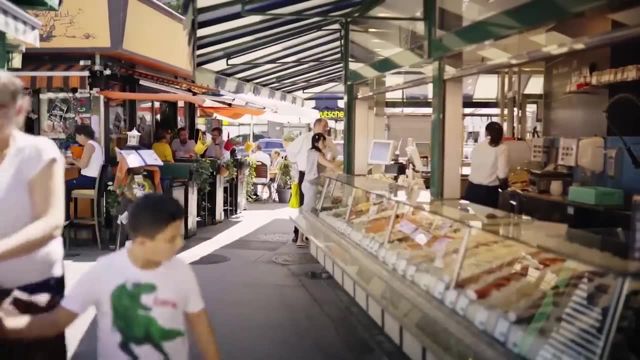 50% of the city is dedicated to this belief, and this green space is spread across 2,000 parks as well as forest and agricultural land. Vienna additionally hosts 135 farmers markets every year, selling food and produce from the surrounding areas, helping residents to cut their carbon footprint by purchasing locally. 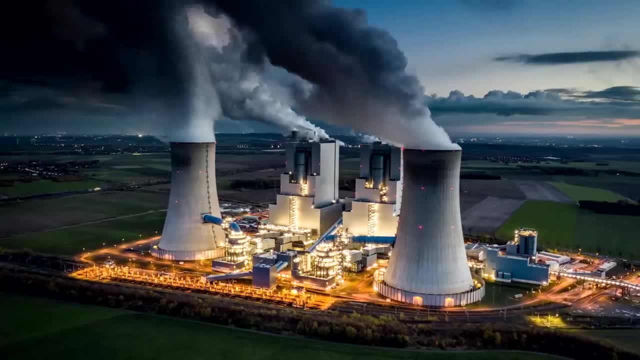 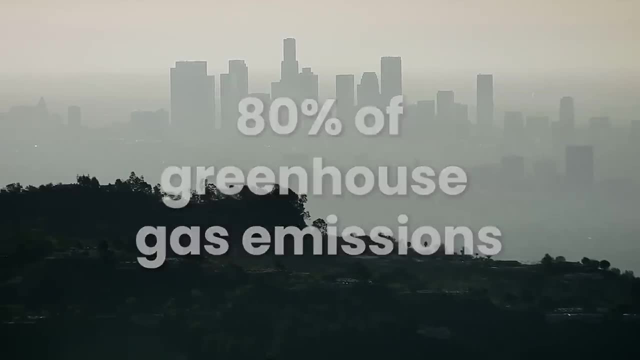 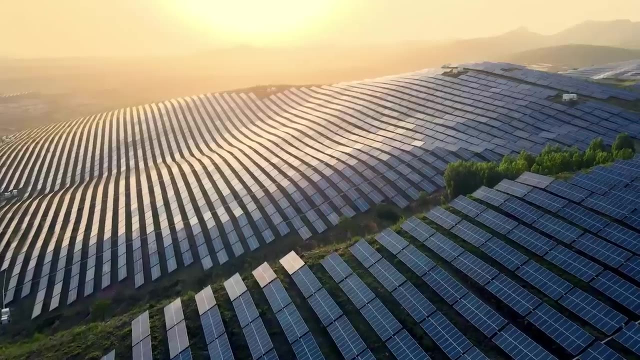 sourced ingredients. Globally, cities consume three-quarters of the world's energy and a responsible 80% of greenhouse gas emissions. The scale and rate of this consumption is a major challenge for both existing and developing cities, But luckily, many locations around the globe are adapting and developing new inventive. 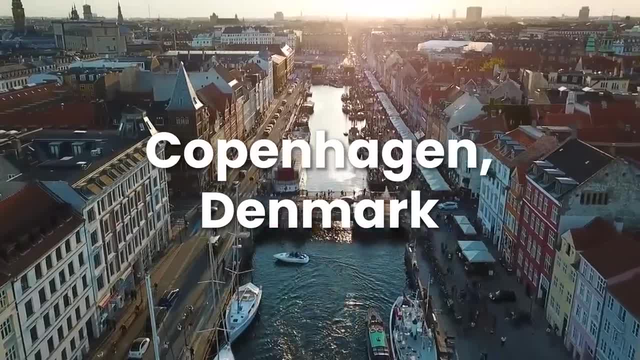 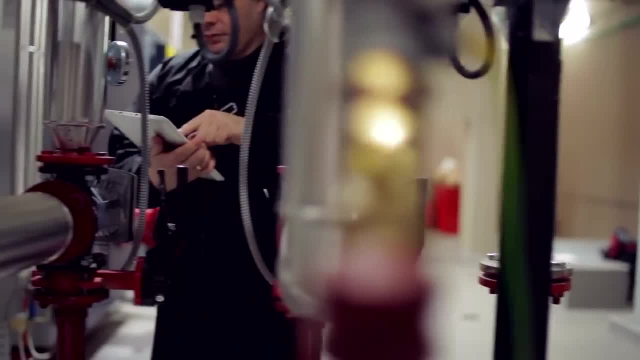 ways to create their energy supply. In Denmark, the city of Copenhagen is leading the way, using its energy supply in smart and sustainable ways, and it's home to the world's largest and most successful district heating system. The system works by capturing the excess heat from electricity production, which is the 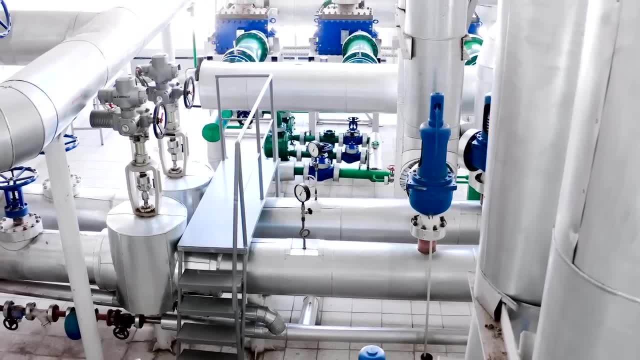 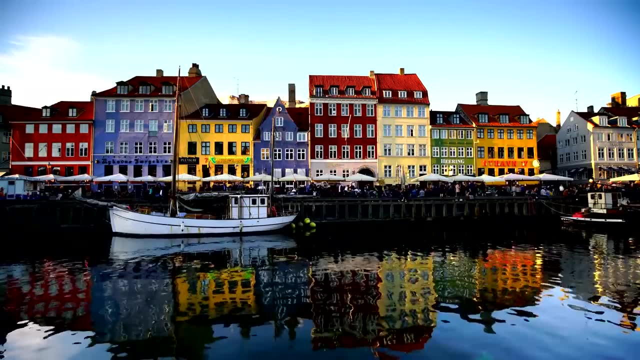 carbon footprint, which is then distributed through a network of pipes delivering the heat to 90% of households within Copenhagen. Additionally, they have also introduced district cooling using a similar system that uses the cold water of the harbour to chill the water that is then delivered to its customers. 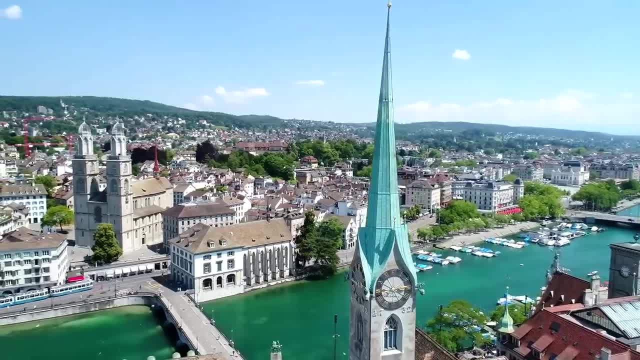 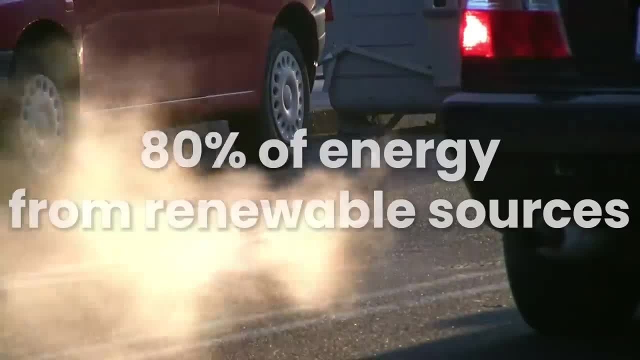 Zurich, Switzerland, has also taken strong measures to reduce its carbon footprint and focus on energy efficiency. The city has introduced tight restrictions on its carbon emissions and, as a result, 80% of the energy utilised by the city comes from renewable sources. 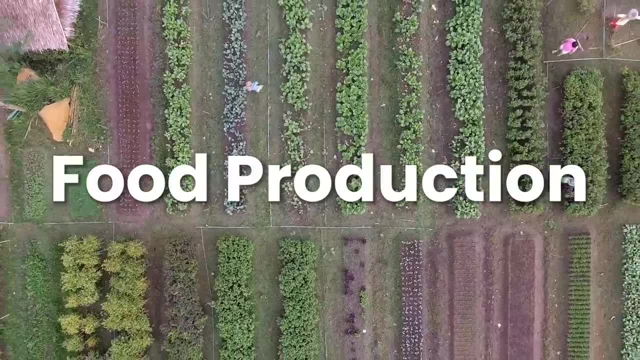 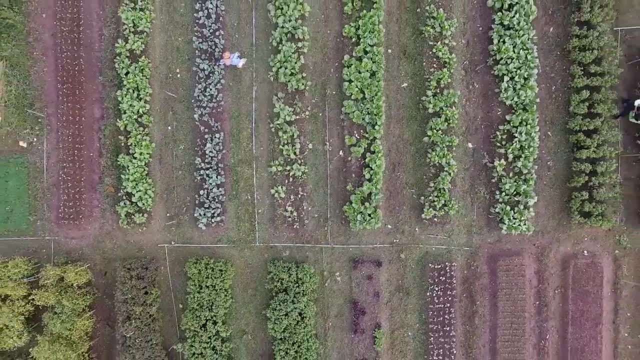 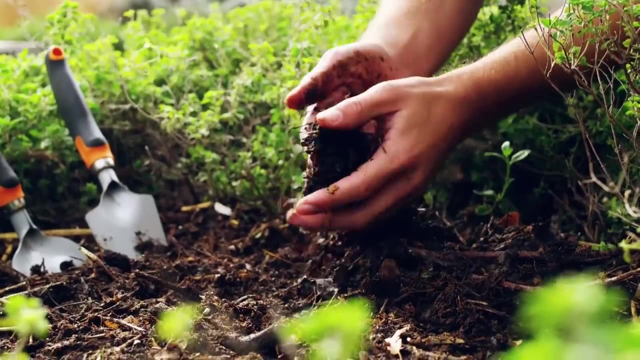 This means that the city's energy supply will be more efficient than ever before. By the year 2050, the world will need to produce twice as much food, whilst reducing greenhouse gas emissions by two thirds, to combat the rapid population growth. In order to do this, cities must find new ways to feed their citizens, focusing on local 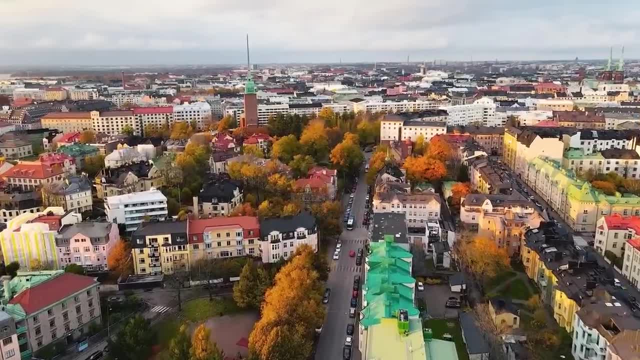 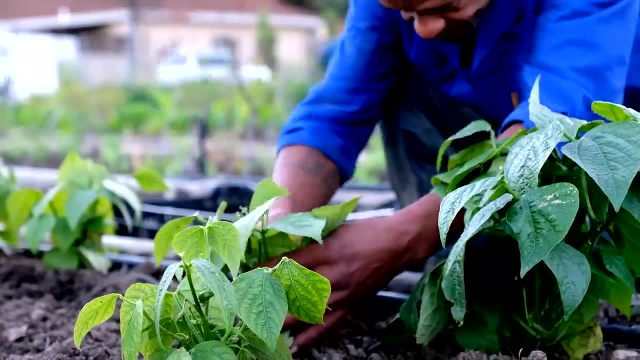 sustainably grown food. Helsinki, Finland, has a rich heritage of urban farming, with allotments dotted across the city, some of which dating back as early as 1918. These allotments can be leased out to residents and the walking paths that run through them. 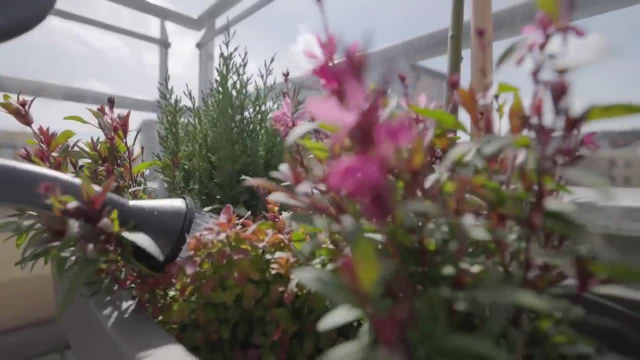 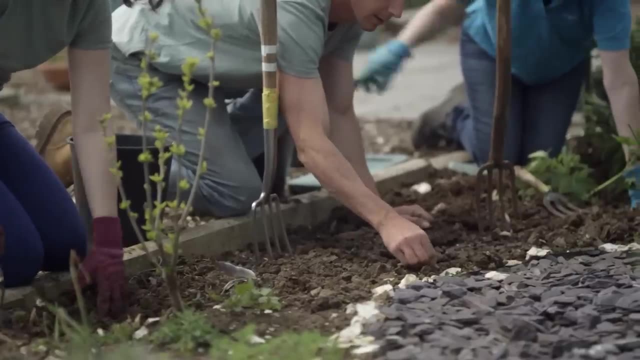 are designated to public parkland. More recently, however, there's been a push for more carbon-neutral urban farming, with residents taking up growing crops on rooftops or even in so-called sack gardens, creating small farming spaces with old industrial sacks. 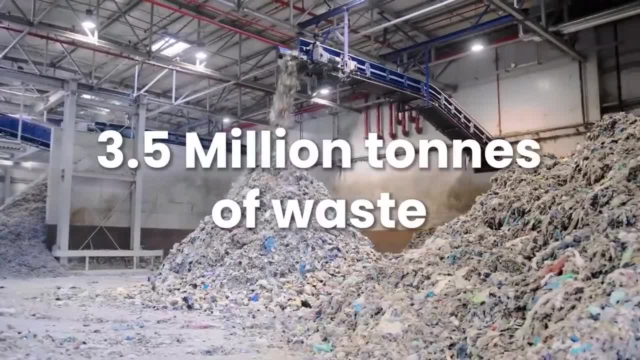 Every day, the world produces more than 3.5 million tonnes of plastic and other waste, which has a direct impact on the health of people and the environment. The world's most important source of energy is the natural gas. The world's most important source of energy is the natural gas, The world's most important.